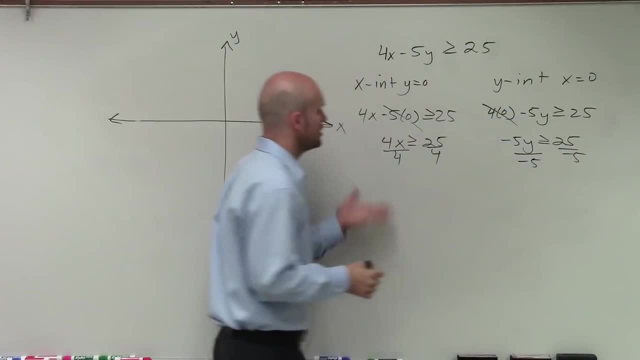 here divide by negative 5.. All right, So now I'm going to have a fraction, but I'm not going to write it. I am going to keep it as a fraction And then to help me graph it, you could use a decimal or you. 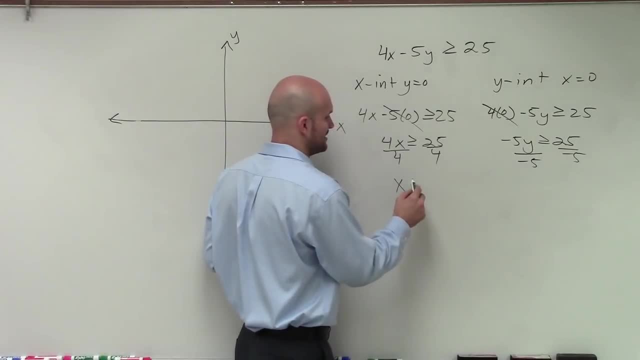 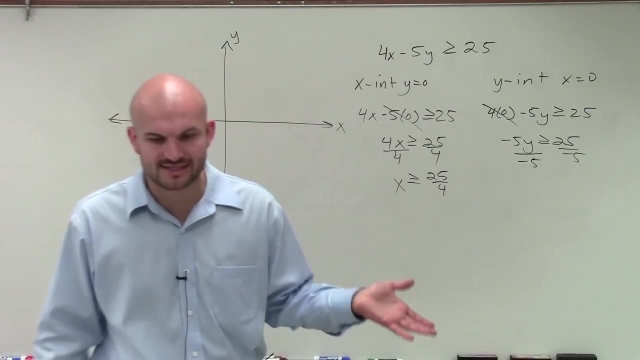 could use a mixed number to kind of help- you find you know- to estimate where that value is going to be. So this is going to be greater or equal to 25.. 25 over 4. And you could go with this as a, you know, as a decimal, But you could also. 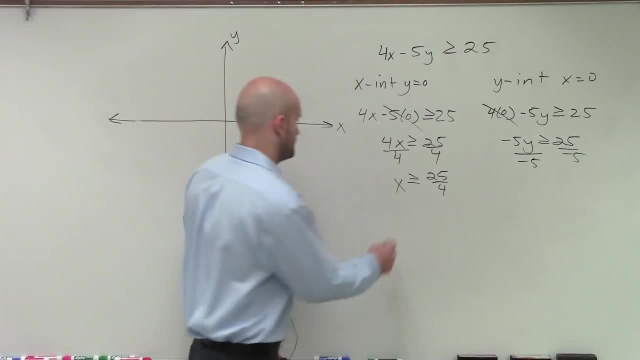 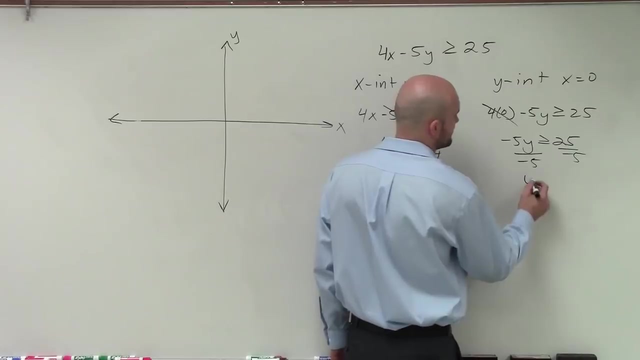 rewrite it as a mixed number, which would be 6 and 1, fourth, or 6.25.. All right, Either way. whatever is going to help you kind of graph it, you could just rewrite that to check it out. Now, over here we're dividing by negative 5.. So remember when we divide by negative. 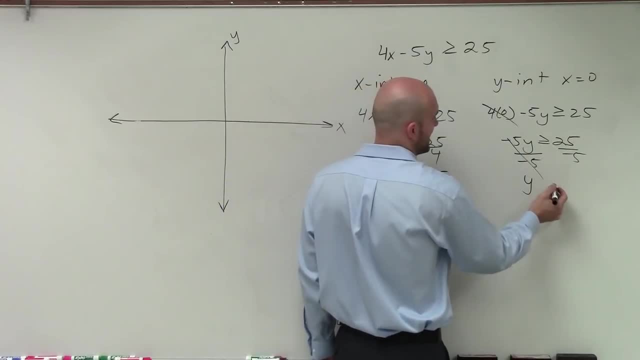 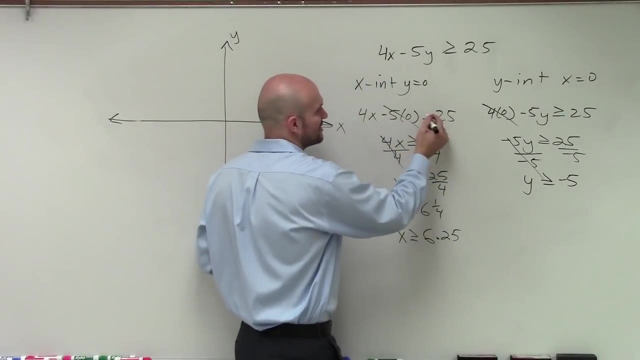 5, those go to 1.. We need to make sure we flip the sign. So that's going to be: x is now greater or equal to negative 5.. However, when solving the x and y intercepts, we're not really going to be concerned. what? 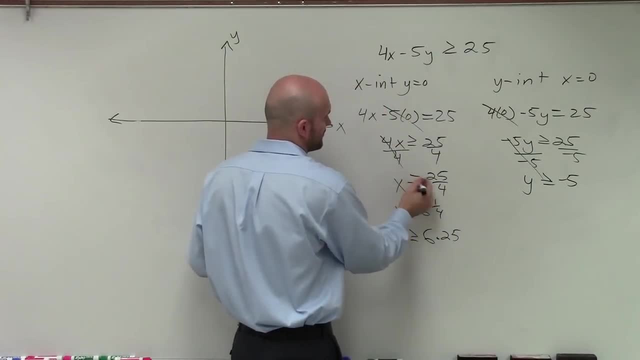 the sign is We're going to show that by using a test point. So I don't even really want to even confuse you so much with that, because what we're going to do is we're going to use a test point to determine where we shade. 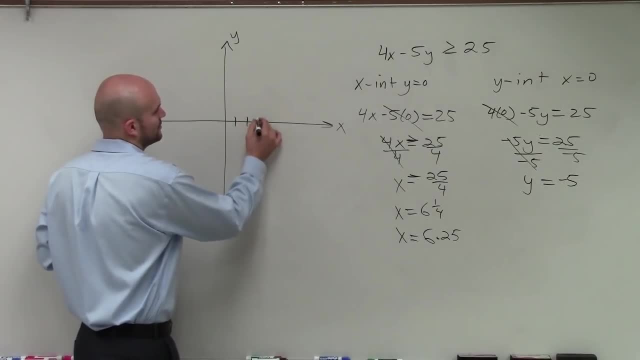 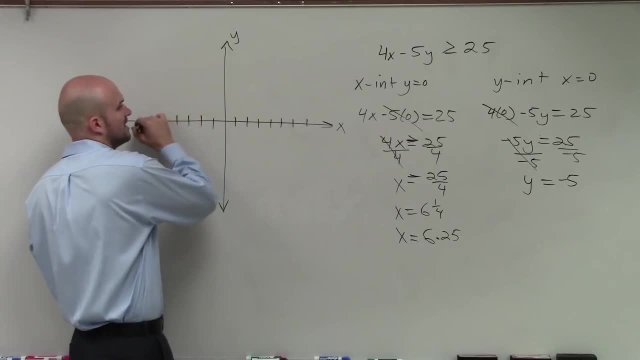 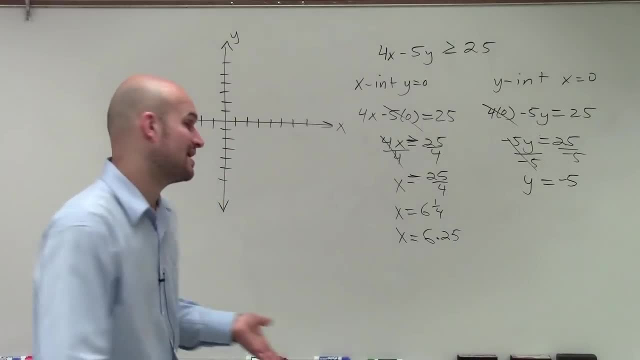 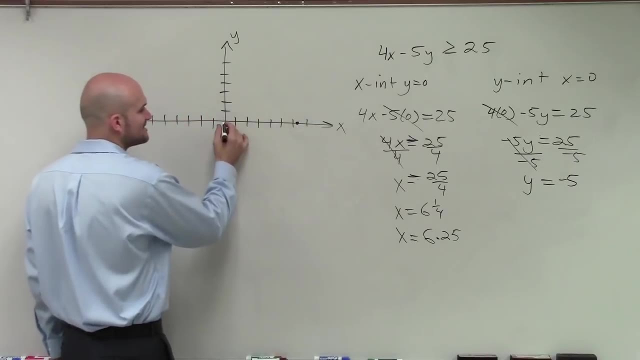 4,, 5,, 6.. Okay, So we say the x intercept's at 6.25.. Therefore, I need to go to the right: 6.25.. 1,, 2,, 3,, 4,, 5,, 6, .25.. And then my y is negative: 5.. 1,, 2,, 3,, 4,, 5.. Okay, So therefore, those. 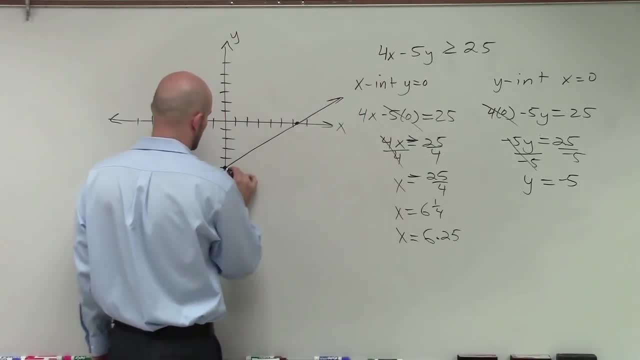 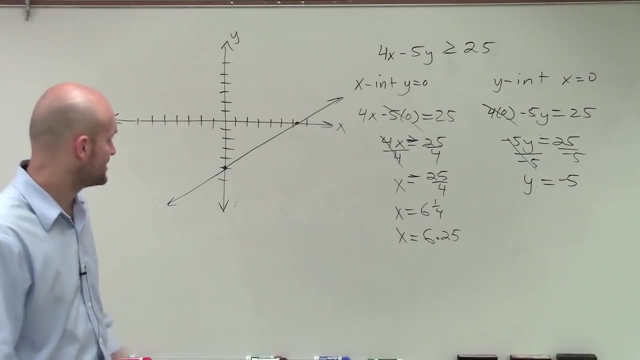 are my two intercepts. So therefore, I know that my graph is going to go infinitely to the left and infinitely to the right And it's going to connect those two points. So I'm going to move up one point And what's going to do is push back my mark and it will connect. 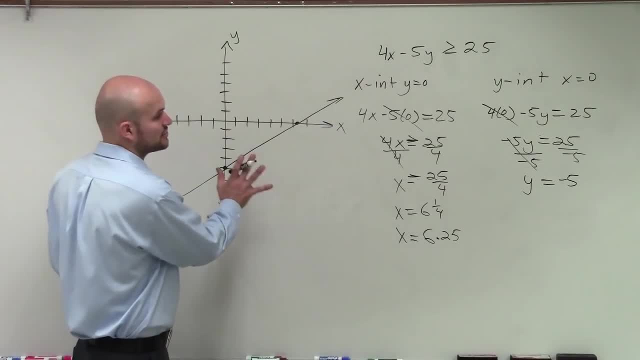 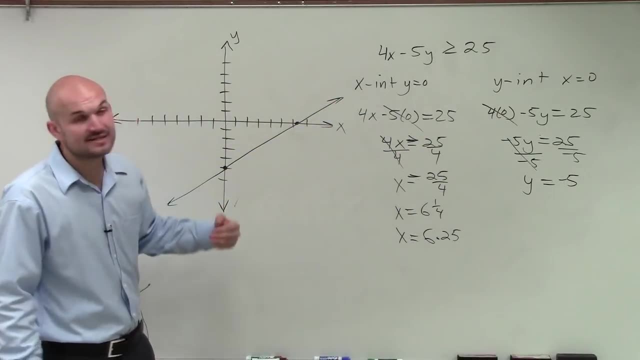 the two points And I know that when I have my mark I don't really have much time to calculate the distance between those two points. So now I know that I have the distance between those two points. So now I have these two points.